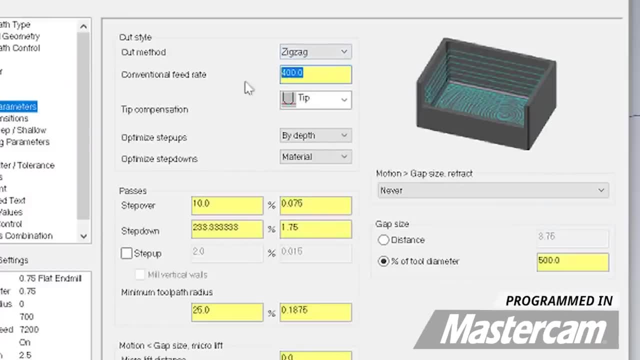 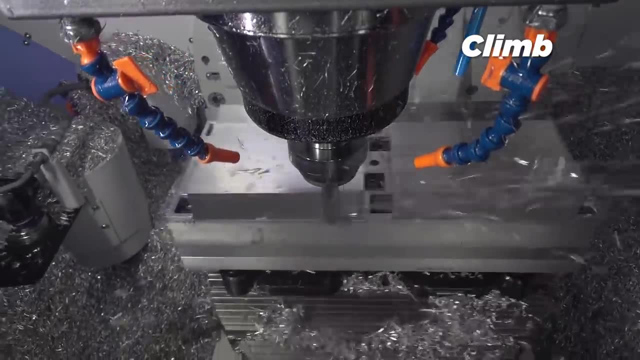 So when you're conventional milling, your tool rubs at entry because you're entering really shallow and then you're finishing your cut deep. So when your tool's rubbing, you're getting faster tool wear and your tool's not going to last as long. Your chip width's starting at zero and then it. 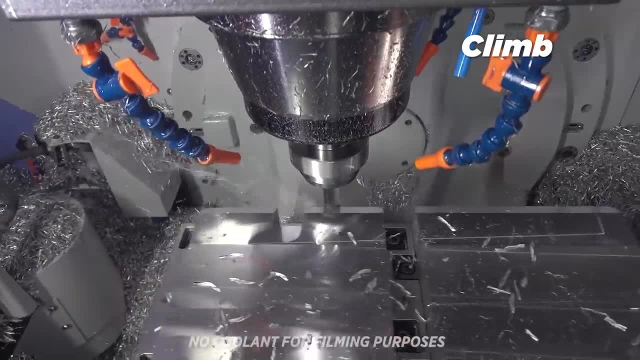 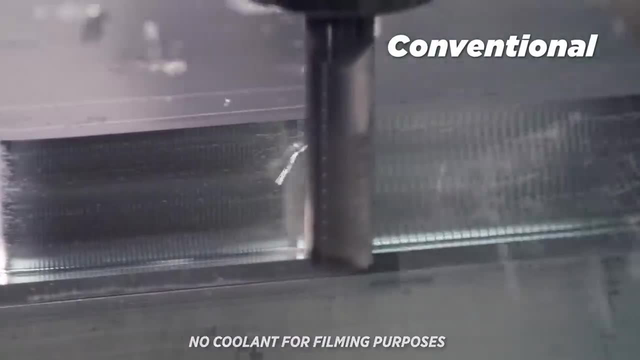 increases. This causes heat Generated by friction to be transferred into your workpiece, which can cause work hardening. In addition to this, you're also going to end up with a worse finish in your part, because chips are being pushed into the path of the cutter, and that'll result in things like smearing. 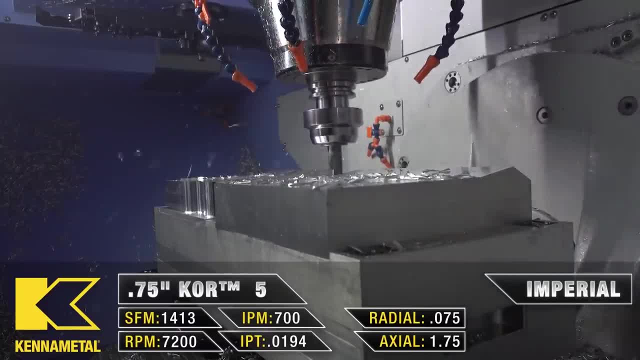 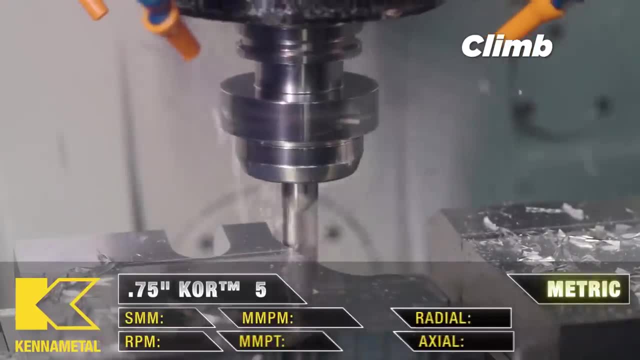 marring, recutting chips. So all these things are undesirable when you're CNC machining. And in addition to these things, which are affecting your tool life and the quality of your part, conventional milling also creates more lift, So it's actually trying to pull your part. 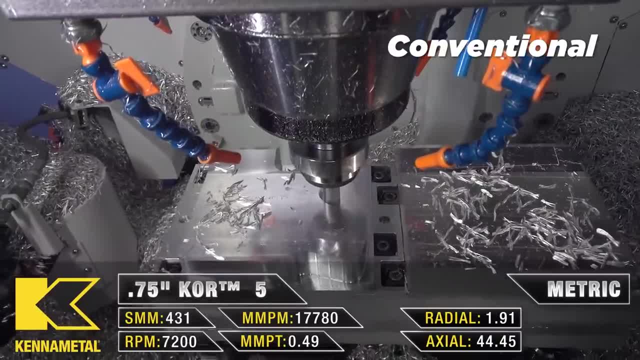 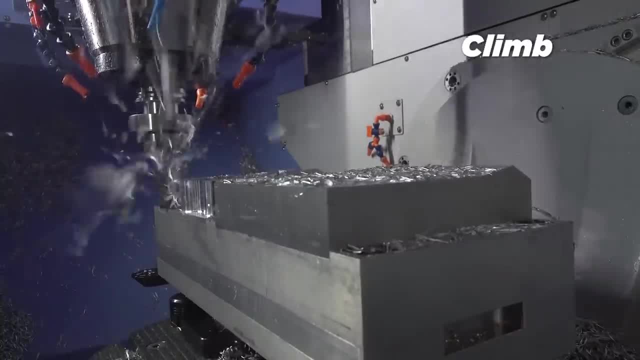 out of your fixturing. In contrast, when you're climb, milling your chip's, starting at maximum thickness and decreasing as you feed your cutter, This pushes most of the heat into the chip instead of into your workpiece. Your cutter's also entering. 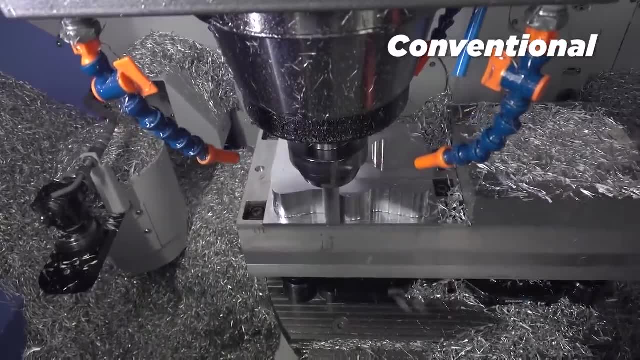 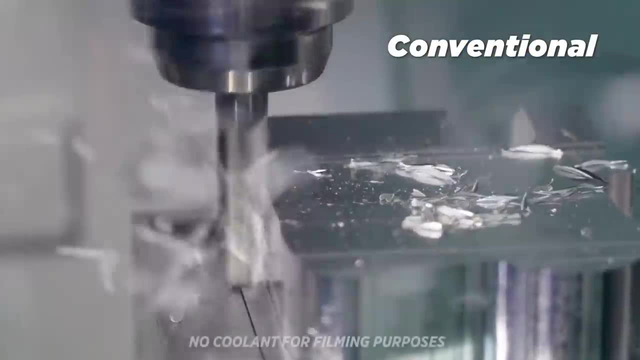 almost perpendicular to the shear plane, which gives you less rubbing, and these two things combined give you better tool life. You're also going to get a better finish out of your part. You know the chips are evacuating behind the cutter now, instead of being pushed in front of. 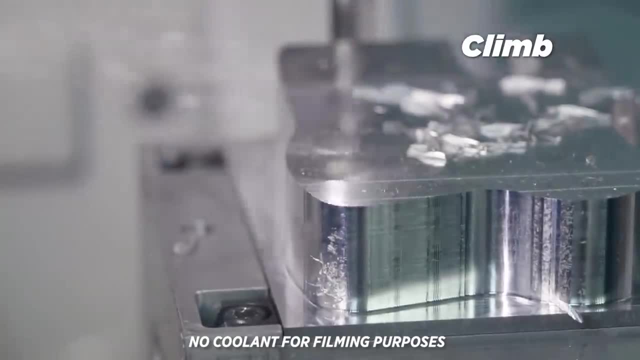 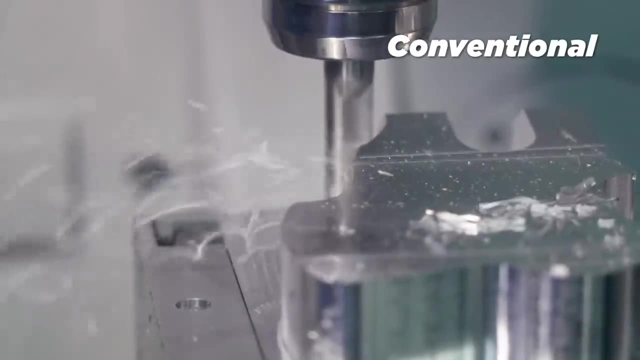 your cutter, where you would get things like the smearing marring chip recutting that you would with conventional milling. Another benefit of climb milling is that, instead of creating lift and trying to pull your part out of the fixture, you're actually pushing your part into your fixture. 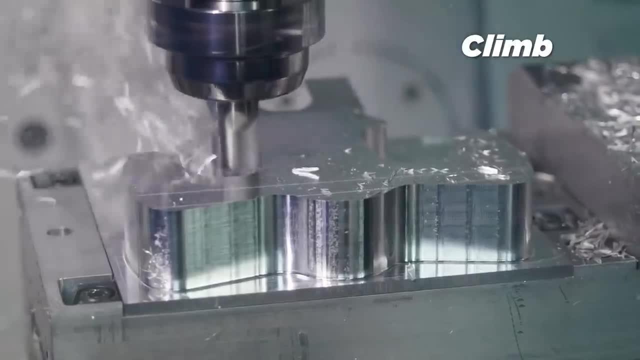 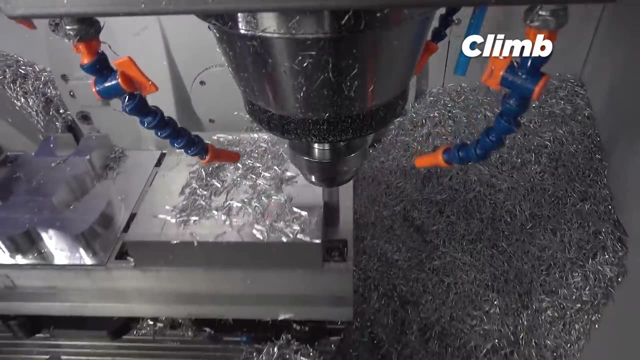 with downward cutting forces. So throughout my career there have only been a handful of times where conventional milling actually helped me. You know, coming from aerospace, I did a lot of tall, thin extrusions, a lot of T-extrusions, angles, and a lot of times these extrusions need. 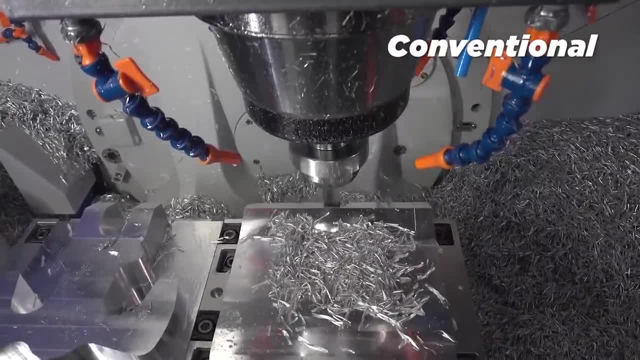 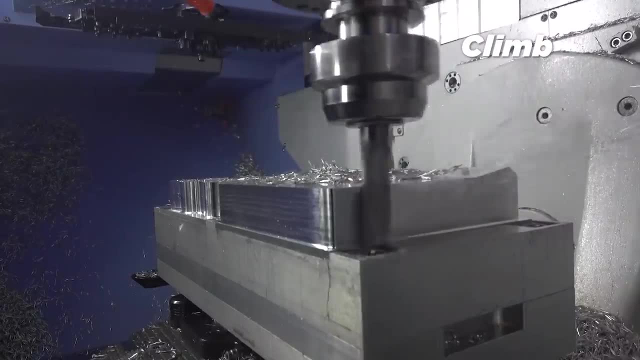 to be cut to length during the milling process. So when you're climb cutting these, the cutter will have a tendency to grab that tall, thin vertical wall of the part and it'll just destroy your workpiece Where conventional milling will provide a lot of room for the cutter to cut. 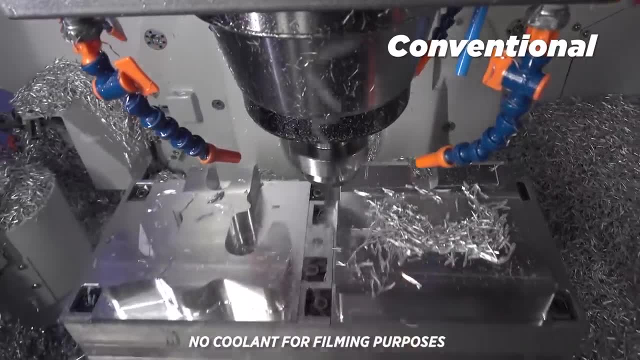 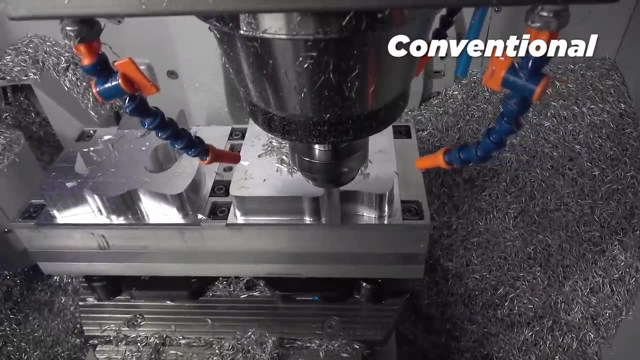 a much more stable cutting condition and you'll be a whole lot less likely to destroy your part. Really, the only other case I can think of is when you're working with case-hardened materials, because in conventional milling, after the very first cut, every subsequent cut is going to start.